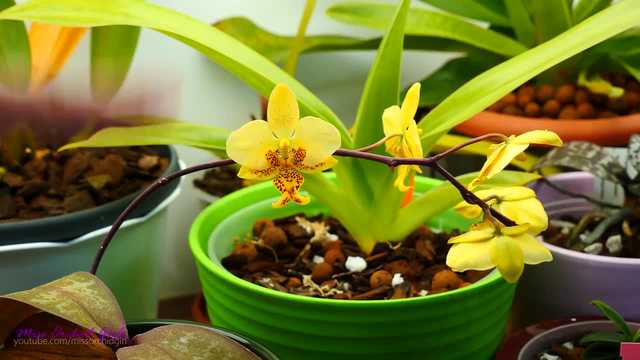 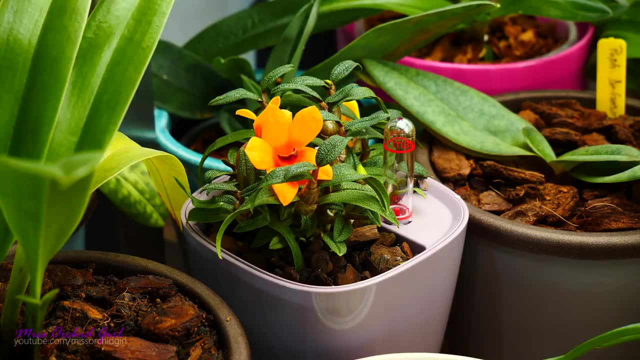 I'll be happy to make one. So today we are going to honor a suggestion and, with that said, let's just start with the topic. Alright, so you might have heard a lot of orchid growers saying my orchid doesn't have available eyes or there is a dormant eye here. Will it develop, Will it not? 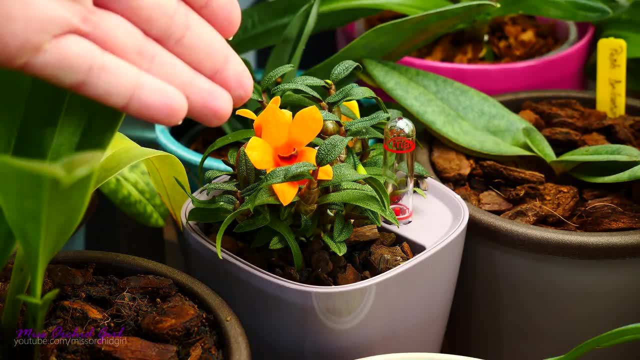 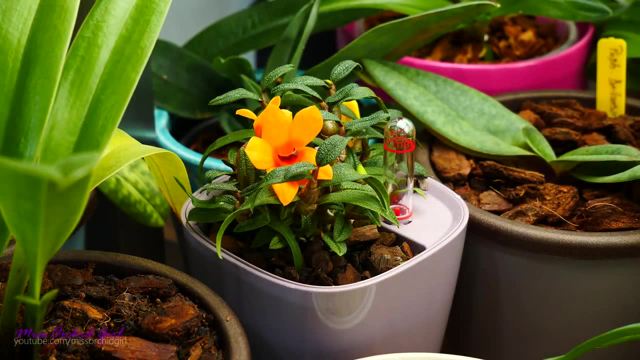 And well, actually these eyes are also called buds, but there is a high chance we're gonna confuse it with the actual orchid flower buds, So for this reason we call them eyes. We could also call them nodes, but typically we do that mostly with Phalaenopsis orchids, because those 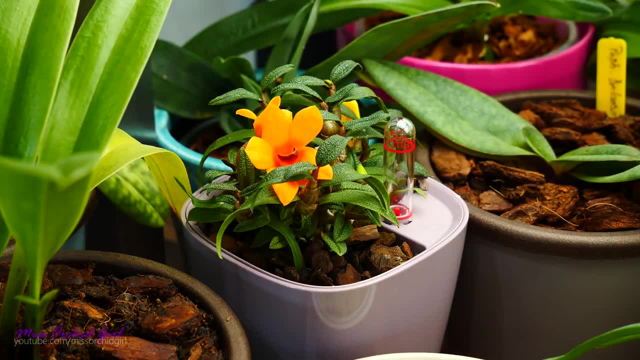 nodes can actually produce something else, which we will talk about in the next video. So if you want to learn more about orchids, you can click on the link in the description below and we'll talk about today as well. The term eyes refers mostly to sympodial orchids, but it could actually refer 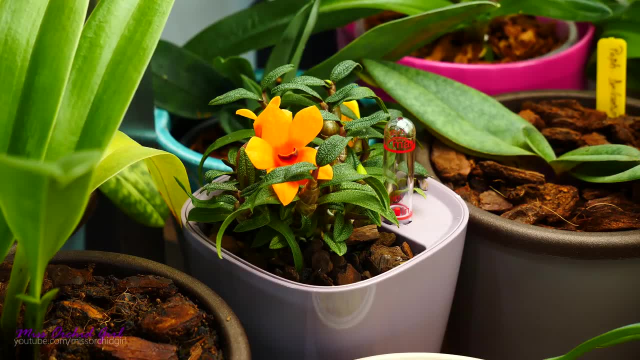 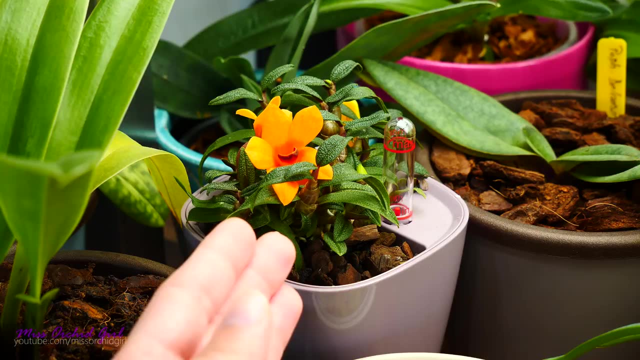 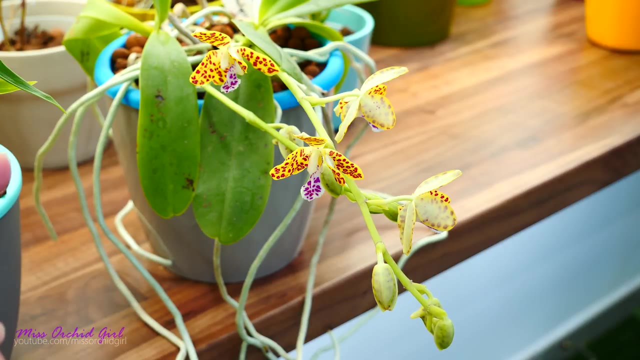 to monopodial orchids as well, And what they are is nothing more than just some growth nodes or buds or formations which can actually create other things, such as new shoots or even flower spikes. We call an eye something we can see, because orchids can actually produce. 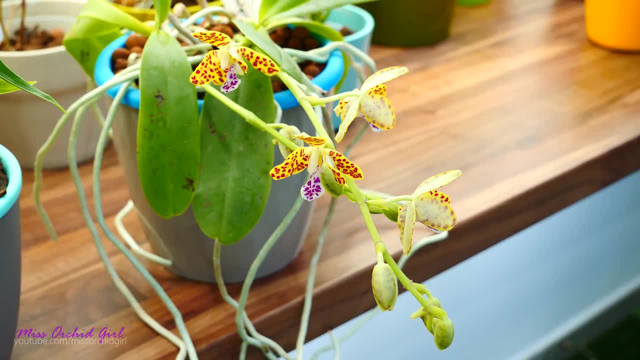 cakies or other structures from places we cannot actually see. Even though there is a growth point or a node or bud there, we cannot actually see it. So in conversation we actually refer to the things we see And I'll give you some examples. don't? 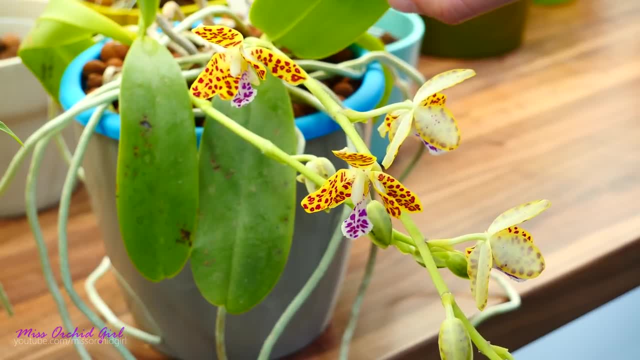 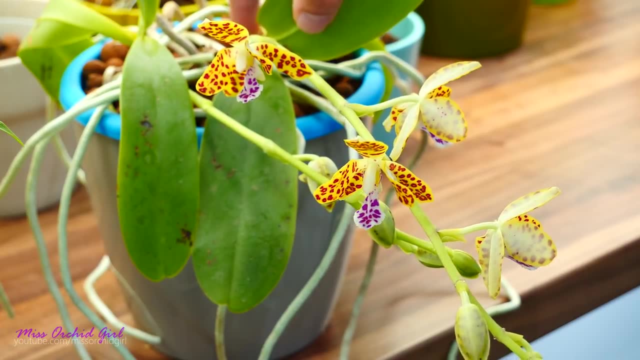 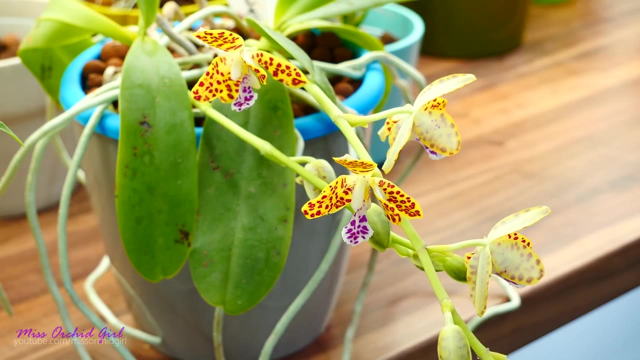 worry. but in this example I have here a monopodial orchid. This is a growth point here in between the leaves, but we cannot see it. so I'm not gonna say, oh, this eye is swelling up, because I cannot see that it's swelling up, but it did produce a flower spike. So in this example I'm not gonna say, oh, 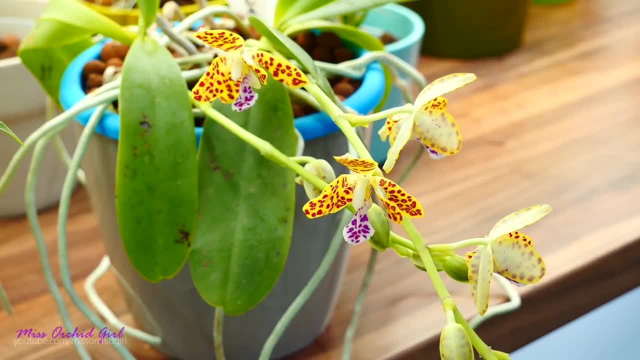 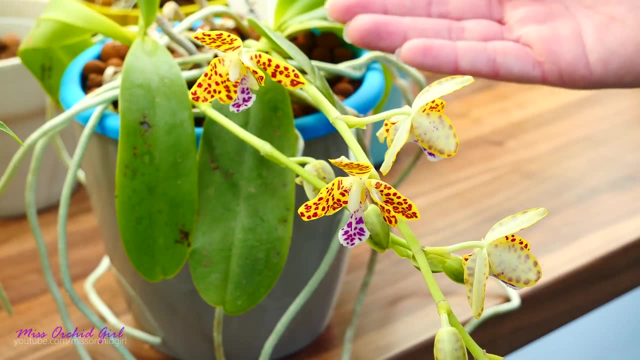 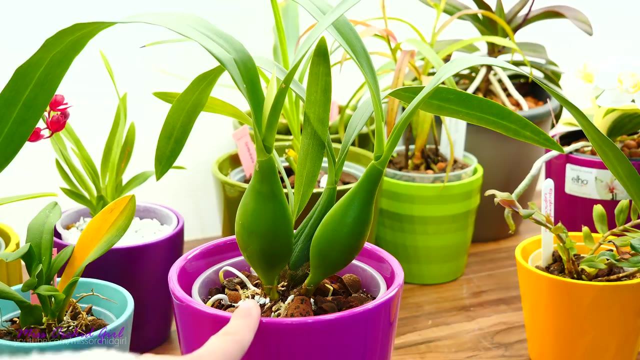 is an eye here. there is an available eye. usually with these orchids, we call them available spaces. this is where a flower spike or a cakey can be produced. what it is is just a growth point or a node, so in this case we won't say this is an available eye, however, on this sympodial orchid. 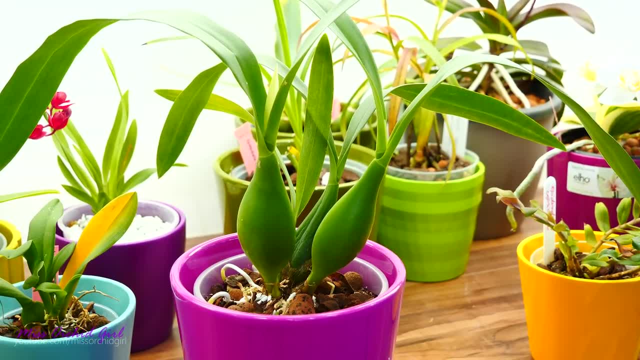 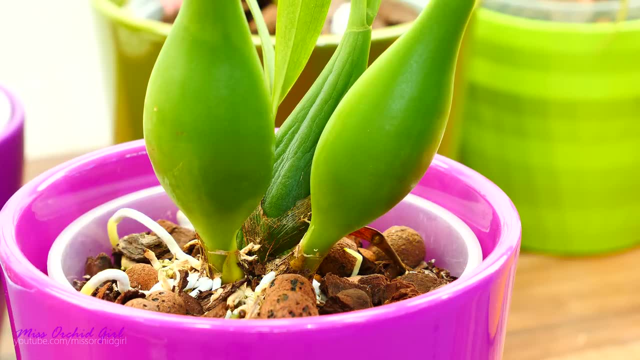 we can absolutely talk about eyes, and let me get you in closer so you see exactly where they are there. they are right there at the base of the pseudobulp. this is a typical location for sympodial orchids, but of course they can vary a little bit depending on the species or variety. 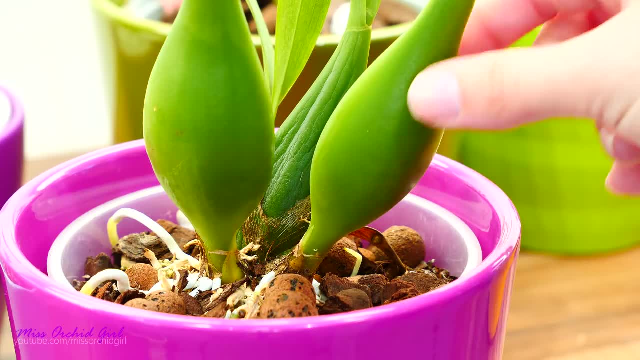 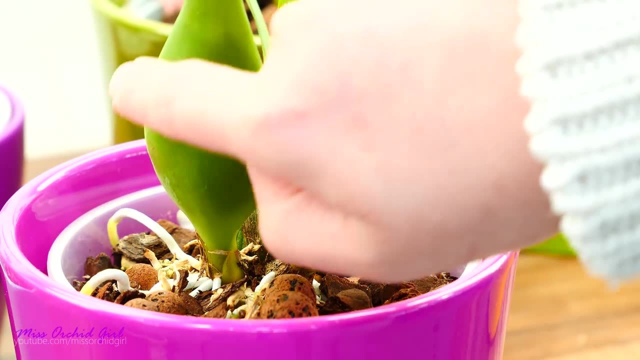 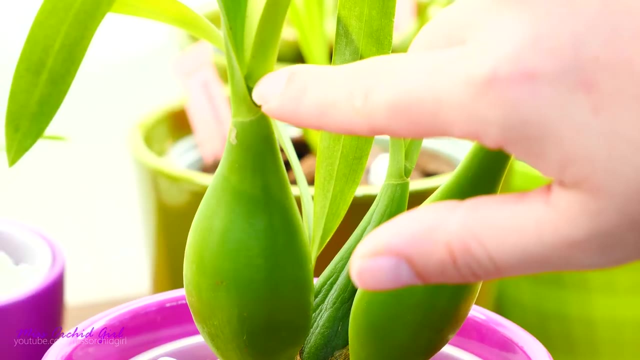 as we will see, most sympodial orchids which produce pseudobulps, they tend to have them here at the base, and this is because the pseudobulb itself doesn't have any other growth nodes on a surface. we have growth nodes here and growth nodes here at the top, but this 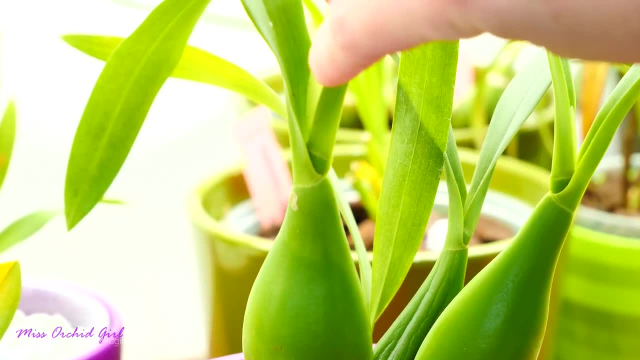 is because when you take the eyes, you want them to maintain that placenta in place. so in most cases you might actually get a lot of sort of a matching ambience between them. and this is important because is where flower spikes usually sprout from. You can see, I have a sheet here. So here at the base, 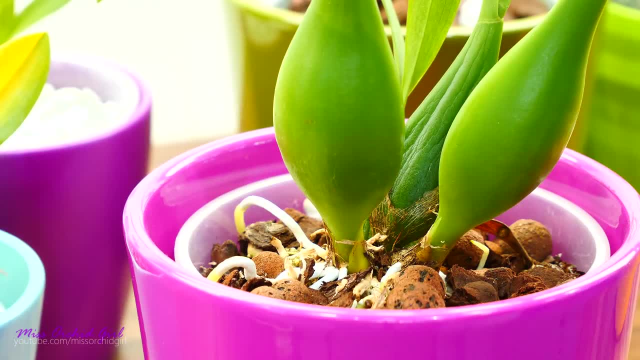 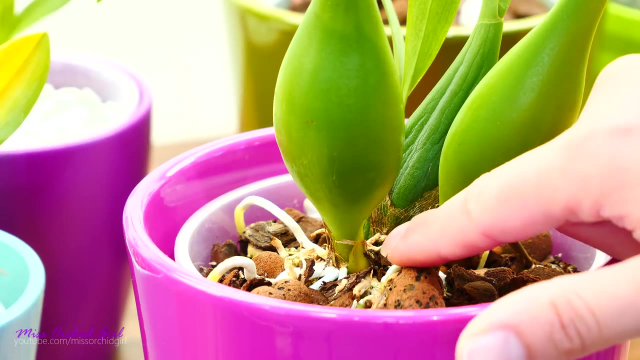 is typically where we are going to see these eyes. Now, if you know sympodial orchids, they have multiple pseudobulbs or structures connected through a rhizome. Well, this rhizome actually continues with each new growth, in the shape of this little eye here, which will start to grow. 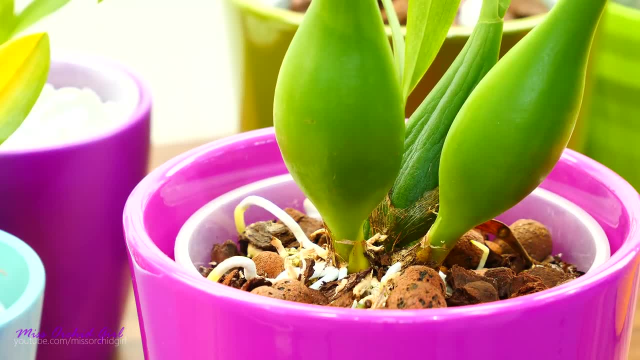 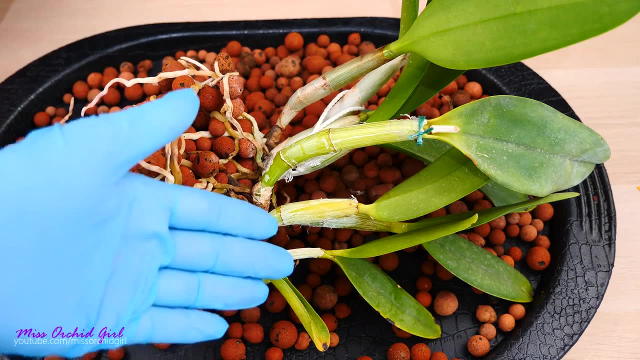 elongate the rhizome and then create another pseudobulb. In yesterday's video we actually talked about dividing the orchid and we took a very close look at the rhizome. If you are curious to actually see the rhizome connecting everything- and you missed yesterday's video- check it down. 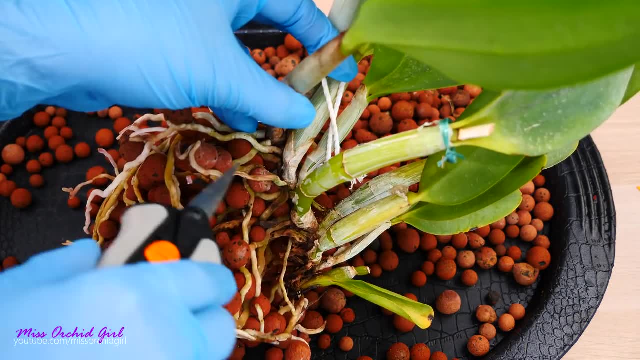 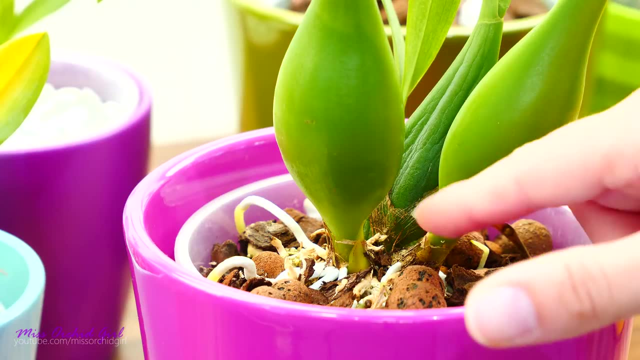 below in the description, I talk more about it. there You're gonna find out how to actually divide orchids. But anyway, that rhizome was created year after year, a little bit more, by these little eyes which continued the growth. Now, how many eyes do orchids have? Well, it depends. 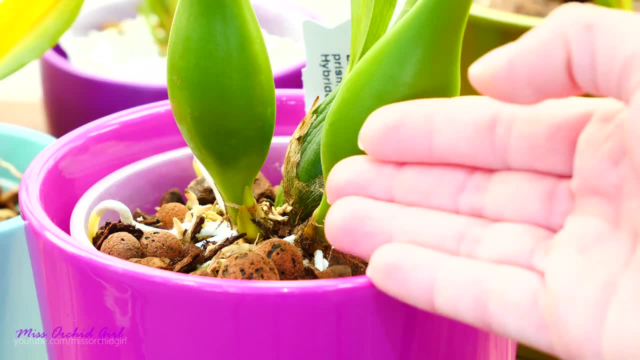 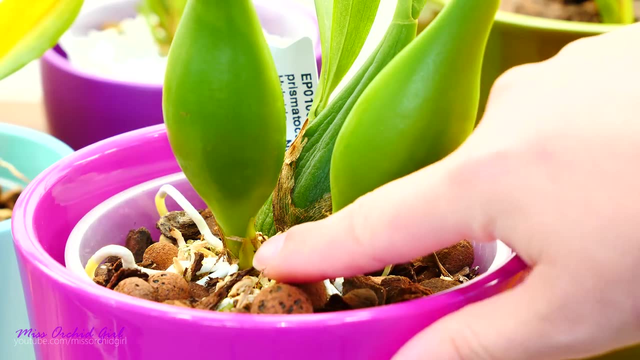 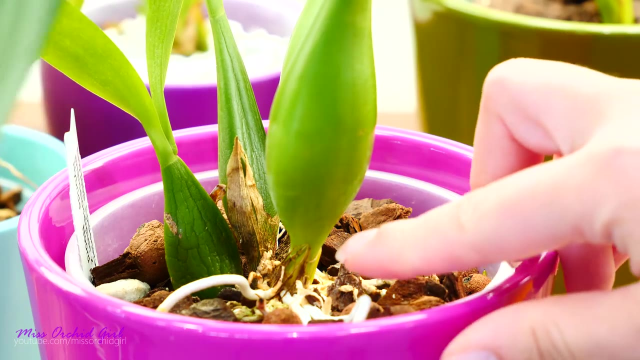 on variety or species. Typically you can have anywhere from two to four or even six available eyes at the base of each pseudobulb. So I have one here, one right above it. right here It's a different eye And on this side I'm gonna have the same. 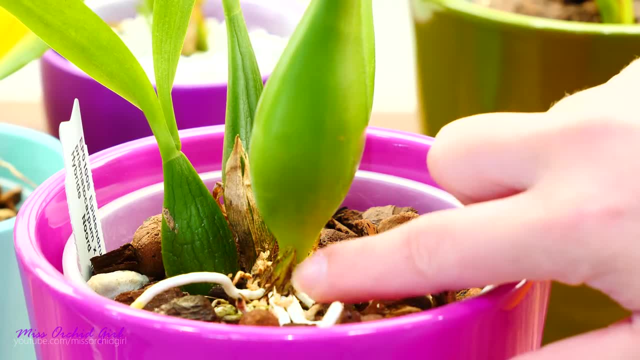 situation mirrored, or theoretically I should, And I know there are some sheets here. but I do have an eye here as well. I'm not entirely sure if I have the fourth eye, It might be right under this one, But again, depending on the species, I could actually only have one available. 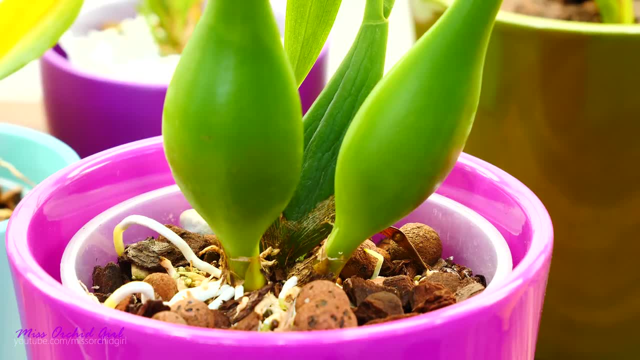 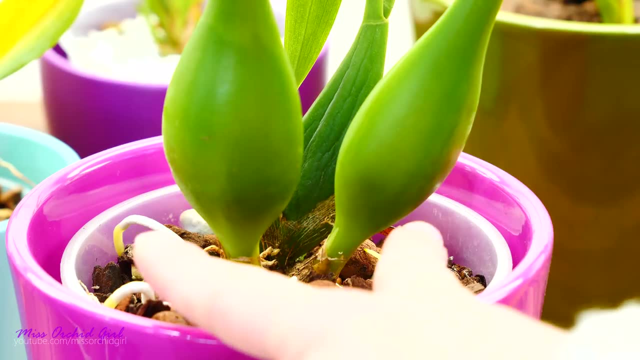 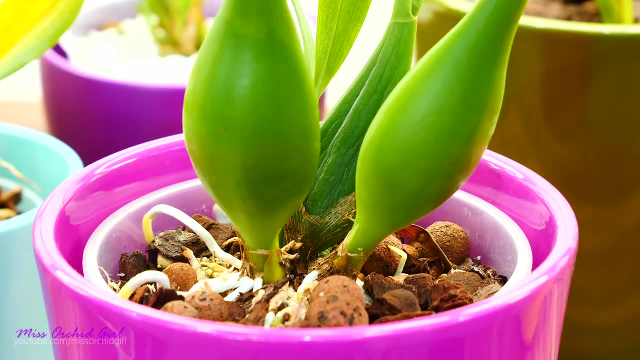 or I could have multiple eyes here And these eyes will at some point develop into new structures. Not all of them necessarily. One of them could develop, Two of them could develop, Like in the case of this orchid. this back bulb here developed two new growths And in rarer cases you can have 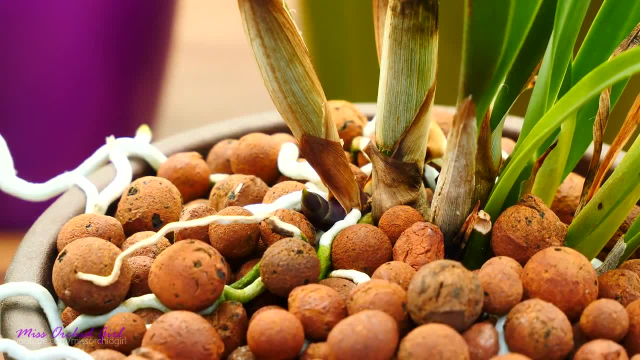 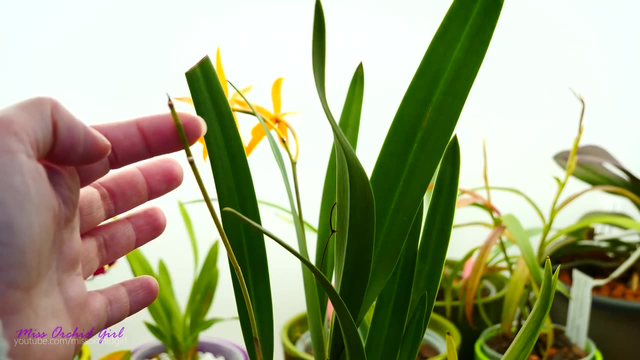 three of them develop at the same time as well. Now, as I was saying, these eyes can at some point start to swell up, meaning they're starting to grow, starting to develop. When will this happen? well, usually when the orchid loses its flowers. So in my case, here you can see, I have a spent. 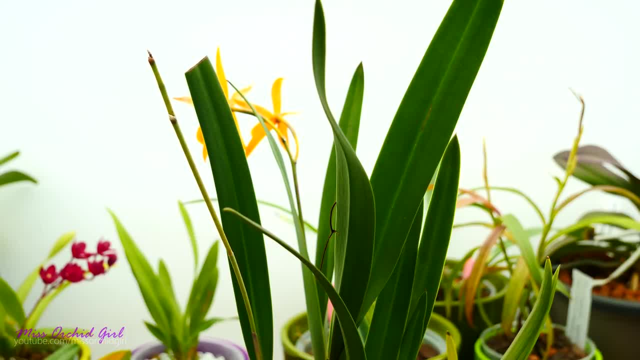 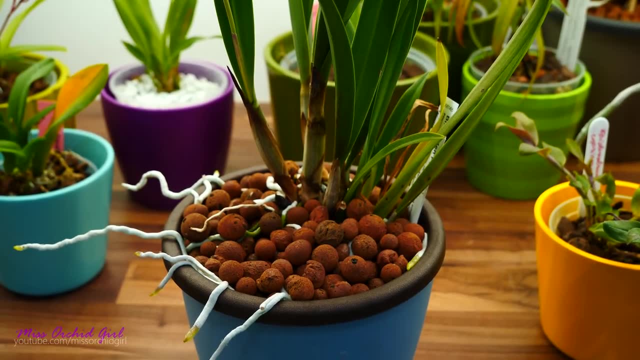 flower spike. There are no more flowers. It is springtime. It is time for this orchid to start growing another pseudobulb, and it will do so typically from the eye of the latest pseudobulb, the one that had the flowers. In my case, I see that my orchid decided only to swell up one of 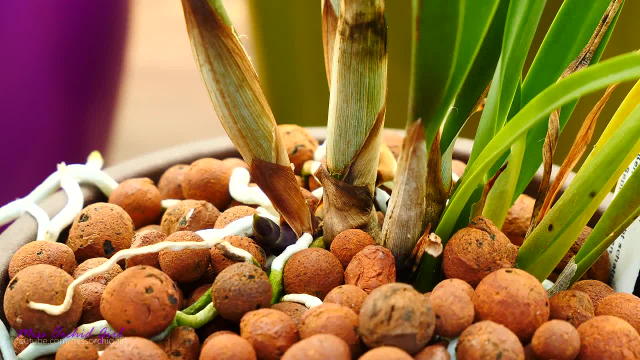 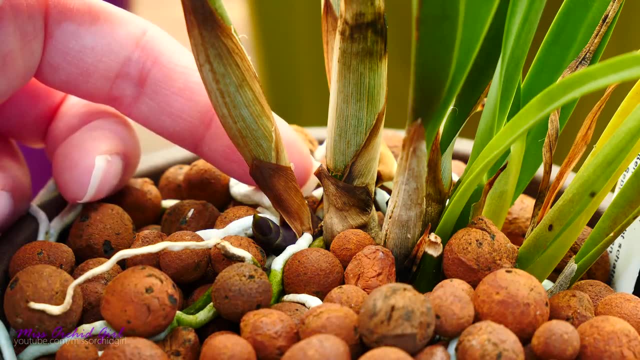 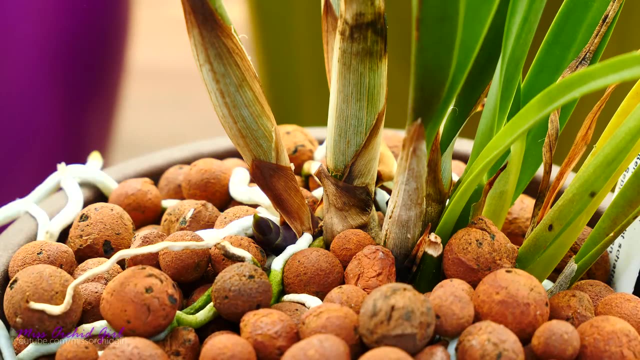 the eyes. That's okay. The funny thing is that in time, even if the rhizome continues to grow, produces more and more pseudobulbs somewhere in the back where you have those eyes being dormant, at some point one of the eyes can just wake up, swell up and create another structure In this. 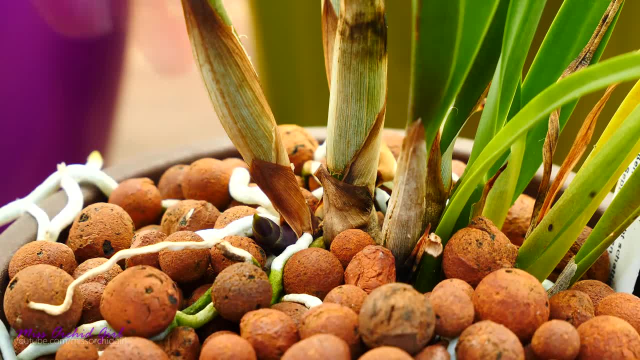 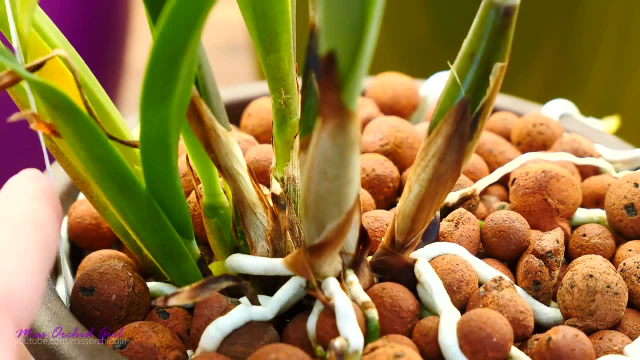 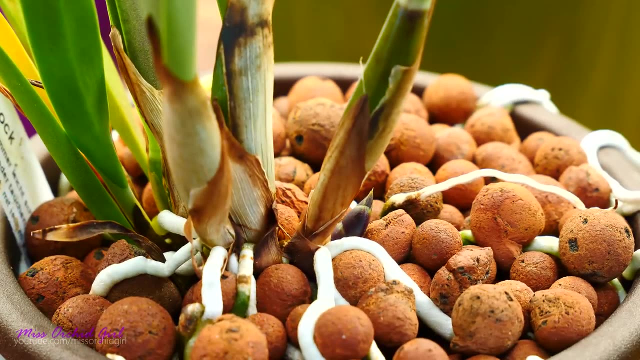 case we say that it created another direction of growth, because, if you can see, here we actually do have a growth direction. We're starting from the back here, with the older structure going forward and the new structures, at least in this case, will always be coming from this. 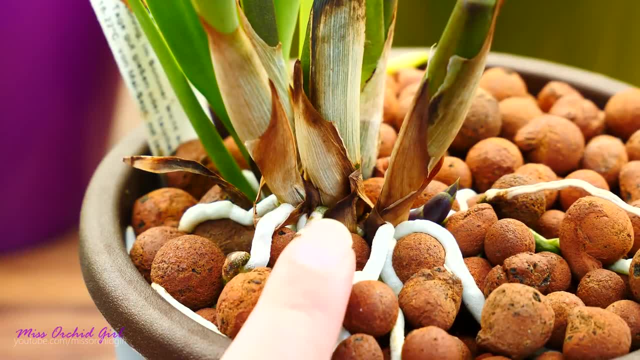 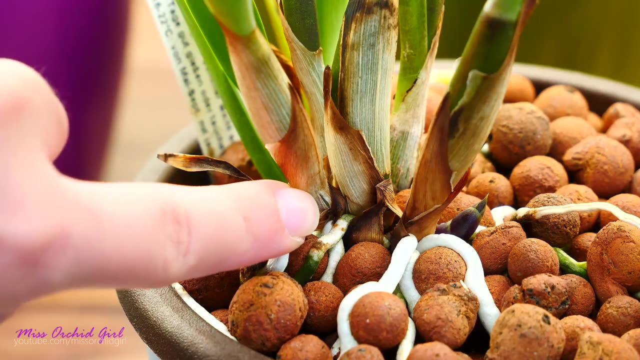 direction. So it can happen that at some point, a pseudobulb will start to develop two of its eyes and we have a sort of fork in the road. If you consider the rhizome as being a road, well, this is an intersection, and I think I do already see something starting to swell here. 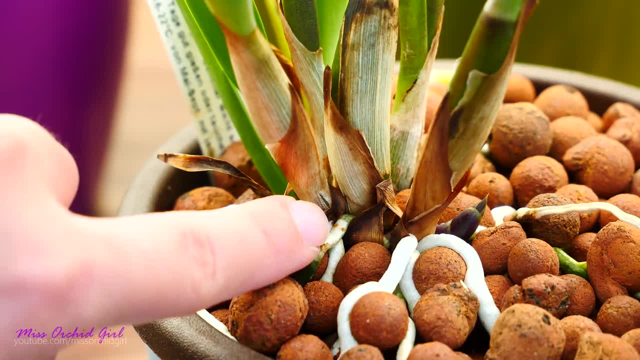 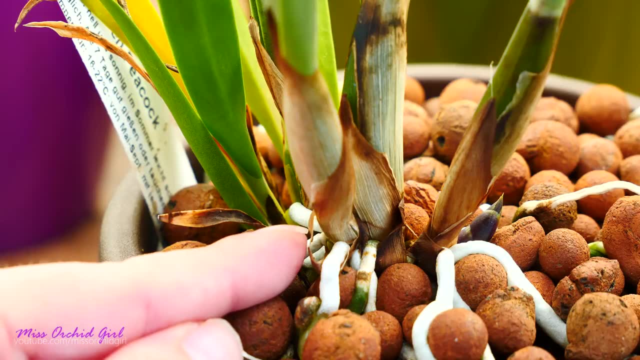 Do you see, the sheath is a little split. Well, I think this node will start to develop. I could have another node, or actually eye developing, here on this side. or I could not, I could have it within two or three years, or I could not Without some hormonal intervention. 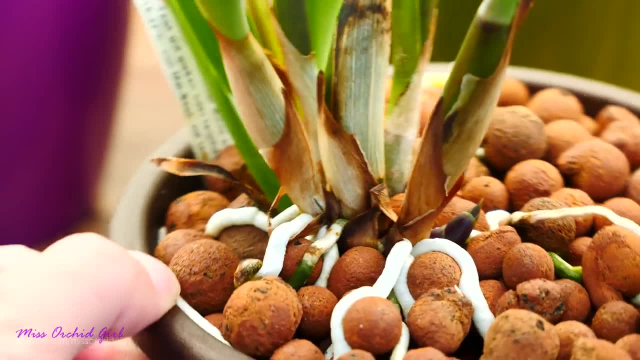 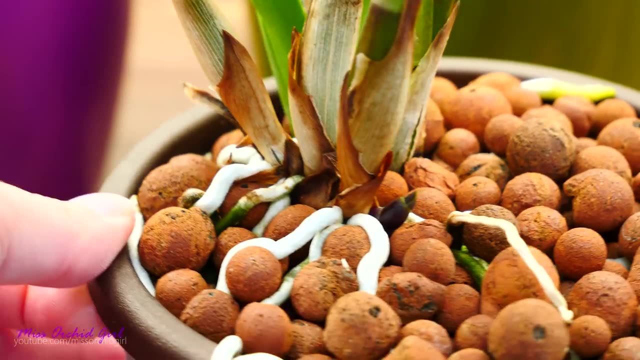 and even though it's a little bit doubtful, you cannot really control which one of the eyes will start to grow. how many will grow? This depends on the orchid. Health has a lot to do with it. The healthier the orchid, the higher the chances you will have multiple eyes starting to develop. 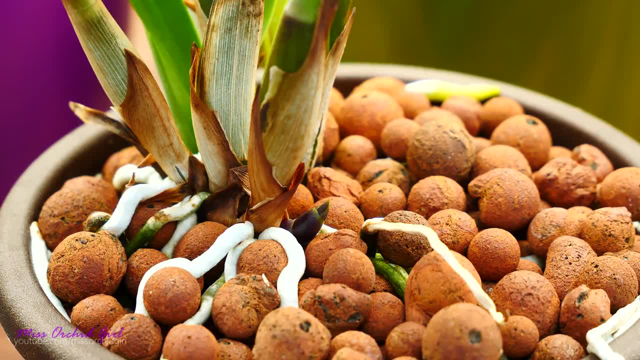 at the same time, But it's not a rule. Even with proper care and proper health, you'll have an orchid which only has one eye developing at a time. you'll pretty much have one direction of growth And that is okay. It doesn't mean your orchid is sick in any way. 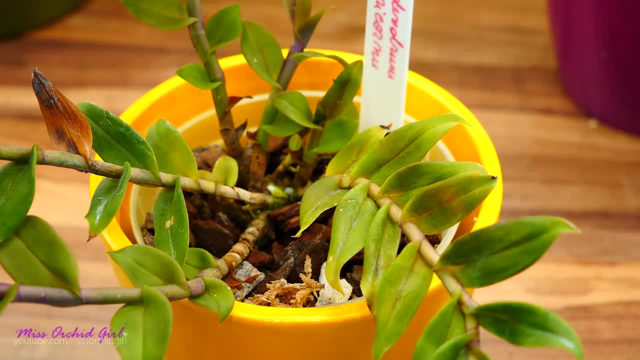 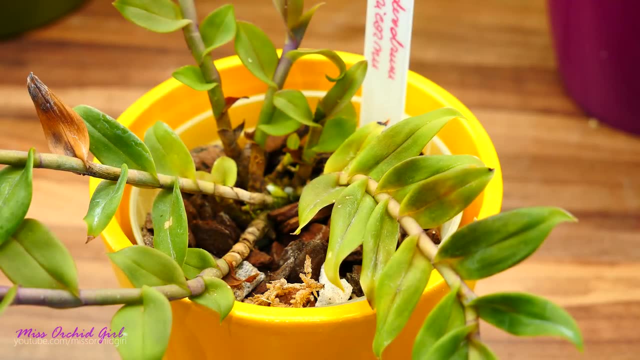 For most sympodial orchids, the swelling up of the eyes means the start of vegetative season or vegetative growth. Typically, this is springtime, But it's not a rule. There are orchids which have continuous growth, which can produce multiple sets of 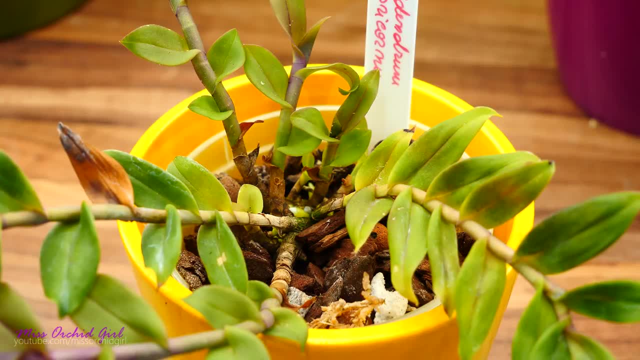 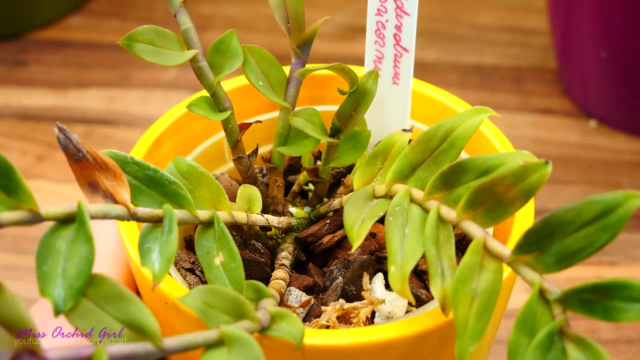 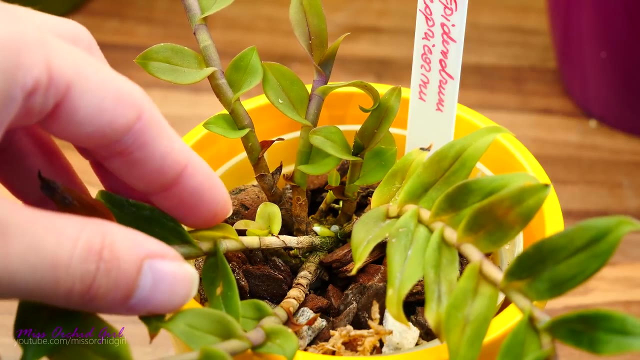 new canes or new pseudobulbs throughout the year, but typically, once an ice starts to swell and form, then the orchid is in vegetative growth. that's how we call it. At this time we need to make sure the orchid receives water, receives fertilizer, because the orchid is actively growing, It produces. 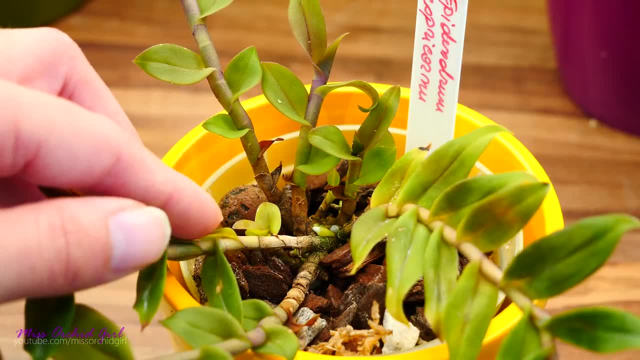 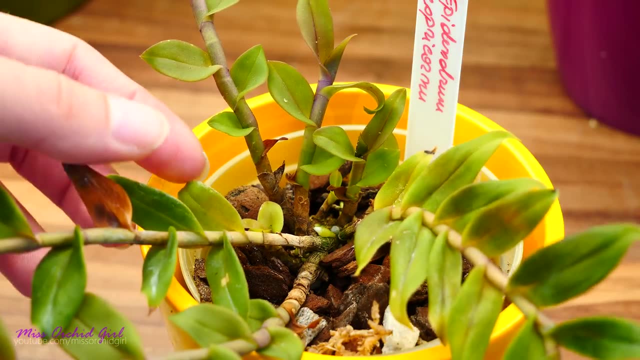 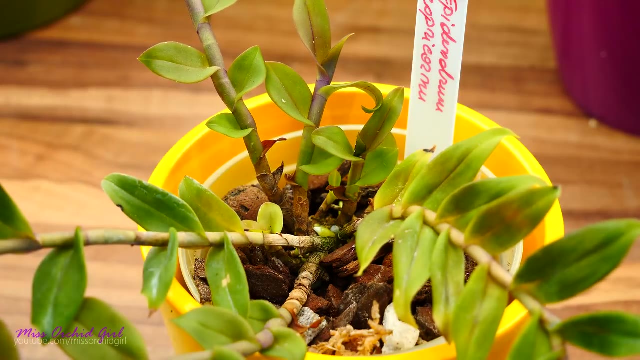 new structures which are vital to its survival and its evolution. Flowers are never vital unless we're talking about propagation of the species overall. but in cultivation we are actually more interested in the vegetative growth to be vigorous and healthy. and all of that because, with vigorous 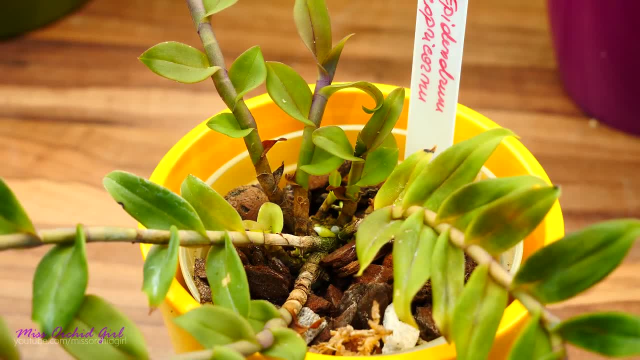 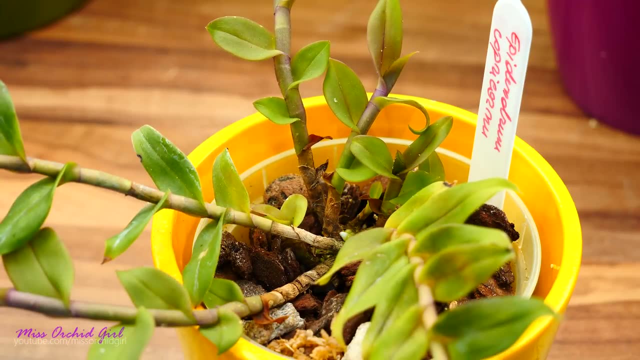 new growth, healthy, good-looking flowers come as well. So, as you can see, we are all pretty happy when we're seeing those eyes swelling up and starting to create little leaves and becoming a fresh new structure, because the more structures we have, the more potential flowers we'll have as 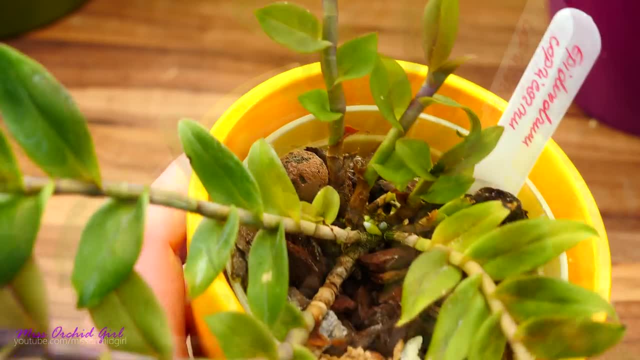 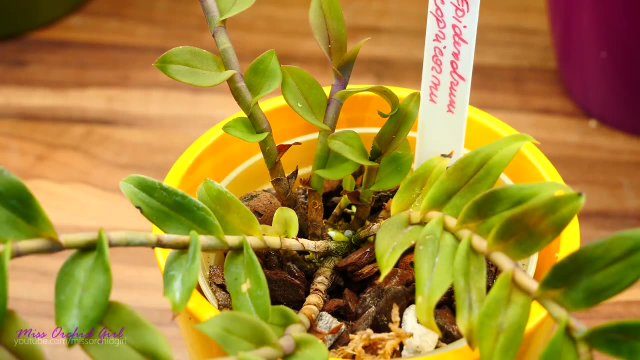 well, the more potential other eyes swelling up and bushing up the plant and so on and so forth. I personally will always be happy to see two eyes swelling up instead of one, because I like bushy orchids with lots of flowers. So up until now we talked mainly about sympodials, which produce. 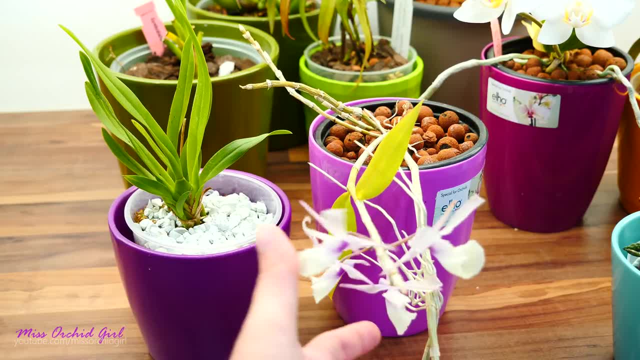 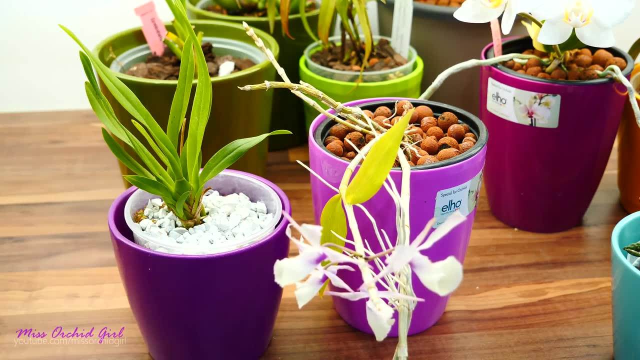 pseudobulbs. but what about those which produce canes? What is the difference? Well, these canes are nothing more than pseudobulbs, but because of their shape and sometimes what they can produce, we kind of differentiate them in conversation. It doesn't mean that they are actually called. 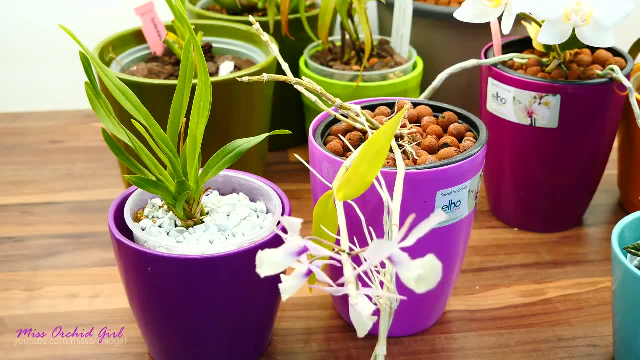 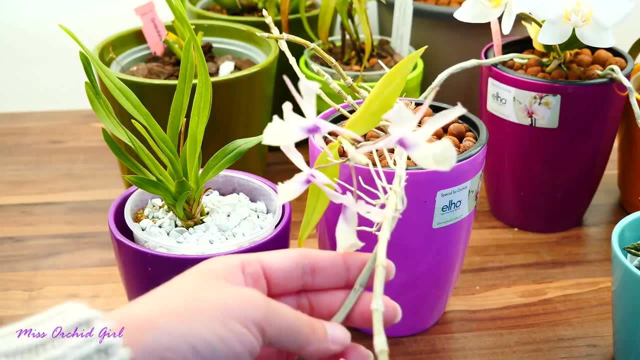 different. No, this is still a sympodial. it has a rhizome, and these are pseudobulbs. They're just acting a little bit different than the ossidium ones and definitely they look rather different as well. So now let's focus a little bit on the dendrobiums. As I was saying, dendrobiums are: 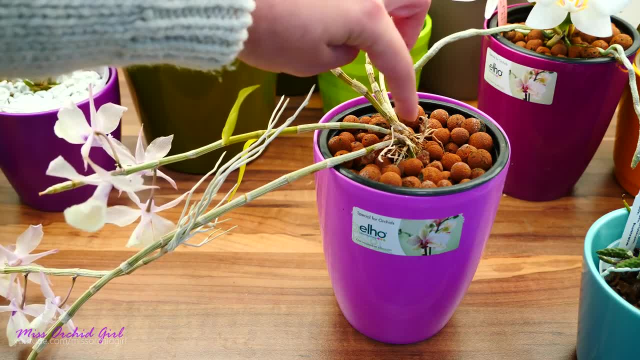 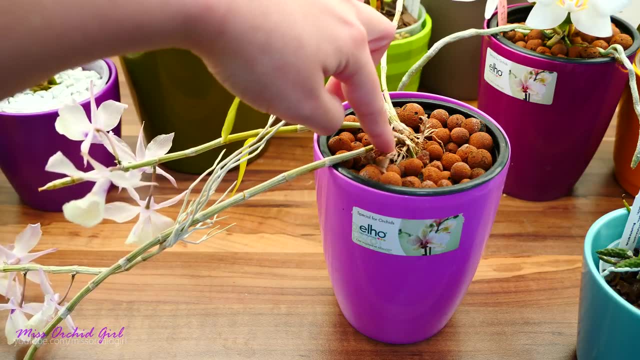 sympodial orchids as well. they have a little rhizome here and each pseudobulb or cane is connected with the other one through this rhizome. Each cane has available eyes at the base, just like the pseudobulbs. 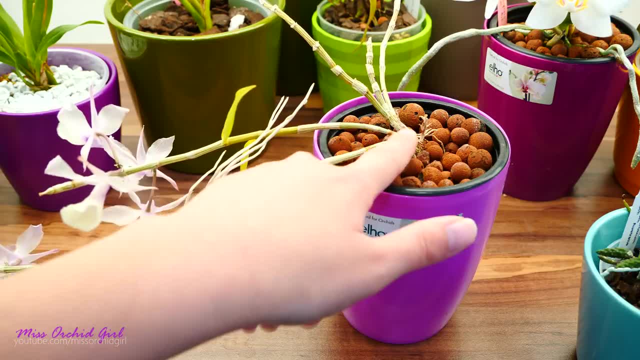 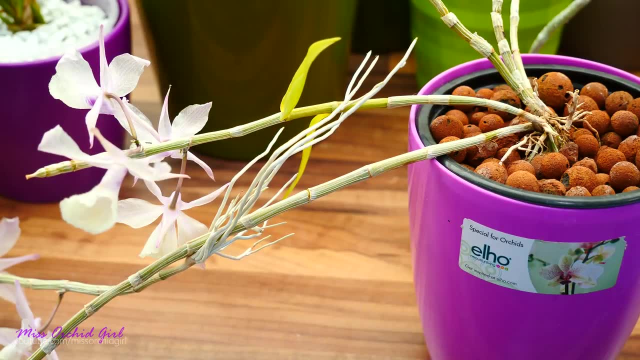 Which will swell up in the growing season, it will create another cane and it will continue the rhizome, Exactly like in the case of oncidiums. What's different is the actual pseudobulb itself. In the case of oncidium orchids, we only had places where eyes could be located at the base. 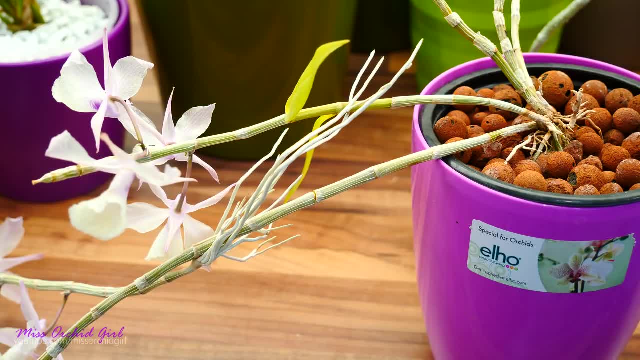 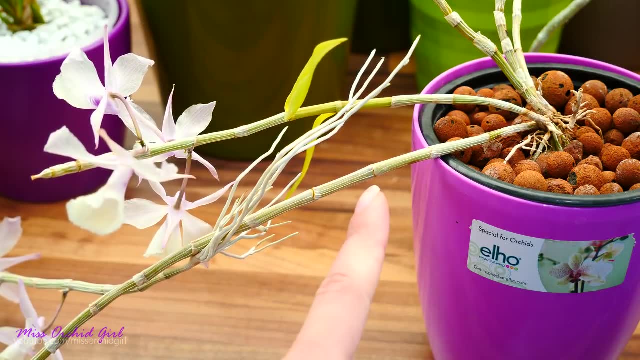 and at the top Well, dendrobiums- at least some of them, have available eyes all throughout the length of the cane. Opposite of the leaf there is a growth bud or eye Which can choose to develop something else depending on the levels of hormones inside. 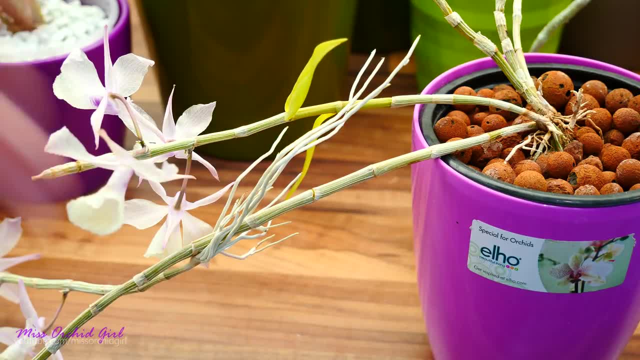 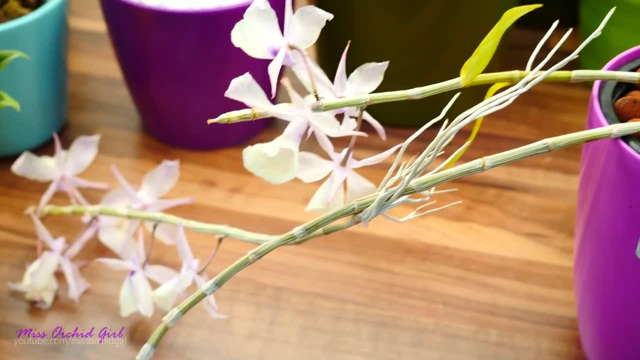 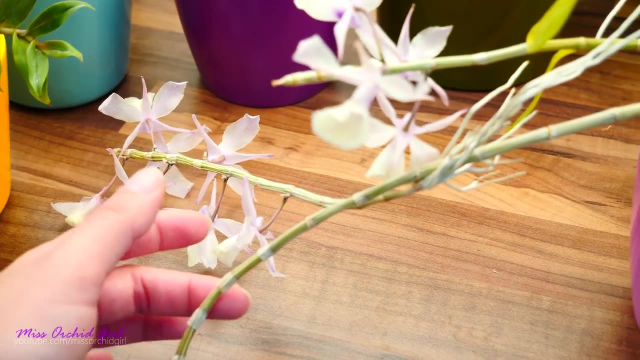 the orchid, which respond usually to external conditions and the weather outside. In my example, here we have a dendrobium which produced flowers at each available eye on its cane, as you can see on this cane here, but also a keiki. This is yet another cane. 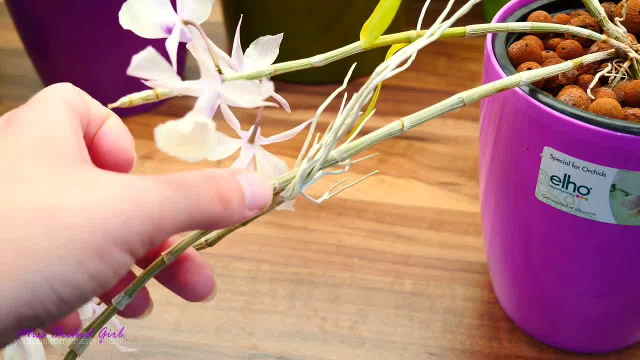 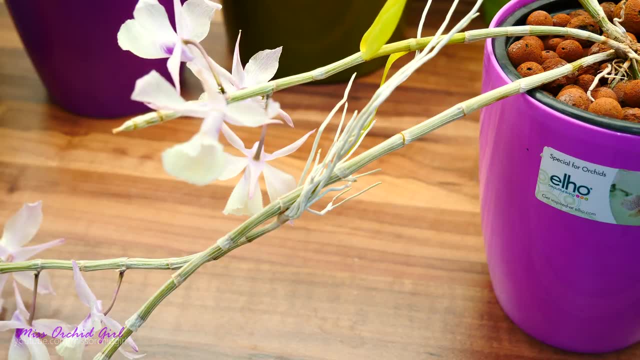 which grew and formed sprouting from one of these flowers. Now, since this is not connected to the rhizome, it isn't actually considered an active part of the orchid. it is rather an offshoot or a keiki. Dendrobiums are those sympodials which typically produce keikis, just like a monopodial, while 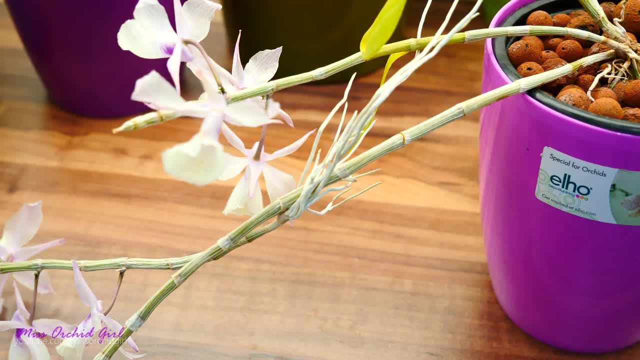 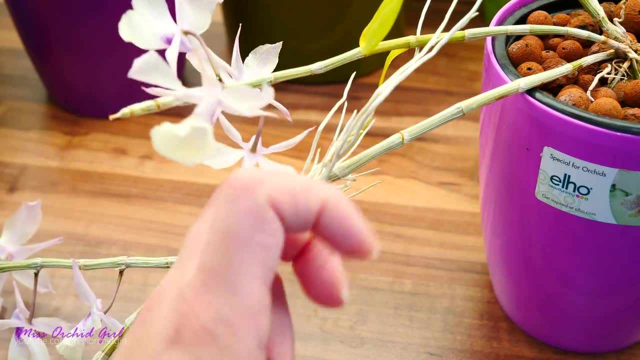 oncidium types and catlea types are not known to produce keikis, Unless we have a hormonal imbalance or things of the sorts. in very rare cases we can find the so-called keikis there as well. But the thing is, dendrobiums can actually be easily propagated through keikis, while 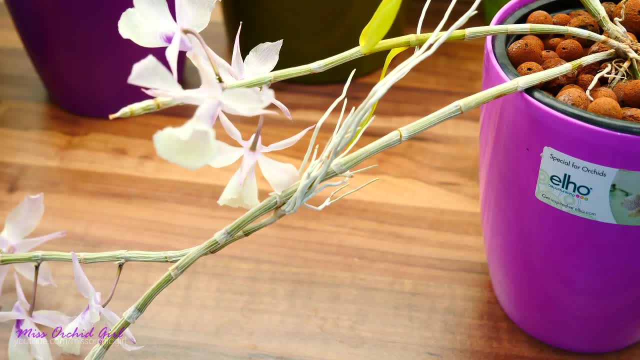 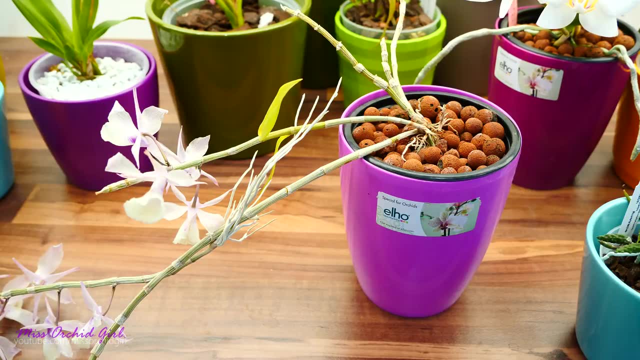 oncidiums and catleas not so much. They are mostly propagated through divisions. So in this case we talk about available eyes, which you can actually feel, but they mean something else. They could mean flowers or other keikis and some orchid growers refer. 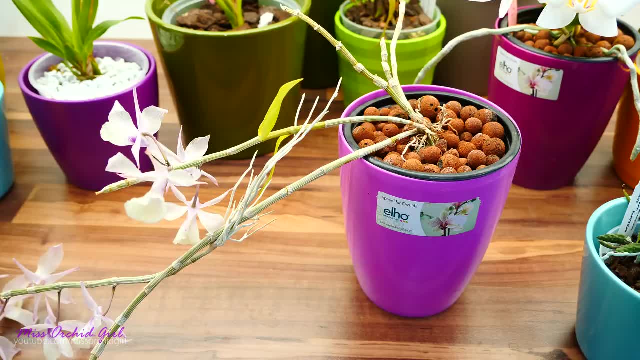 to them as nodes rather than eyes. just to differentiate between the basal growth points and the actual suitable growth points, Some people call these eyes as well. This is not scientific vocabulary here. it's just informal talk between orchid growers, so things can get a little mixed up. 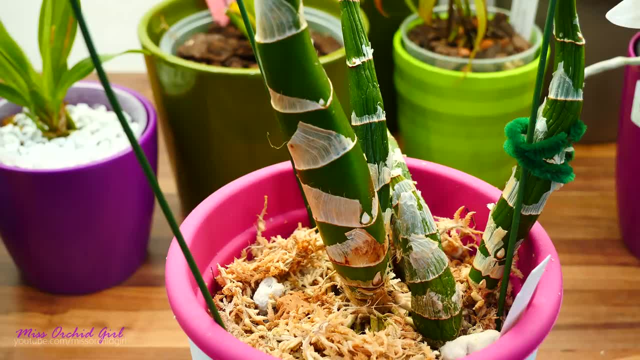 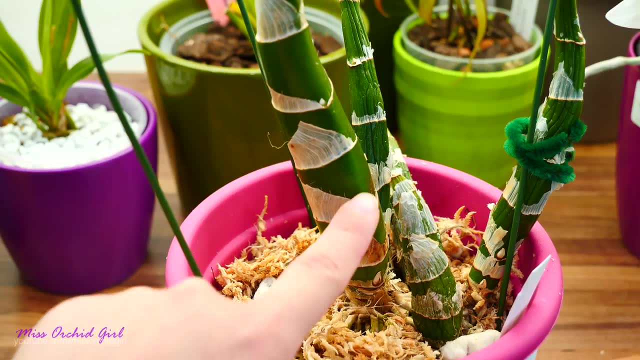 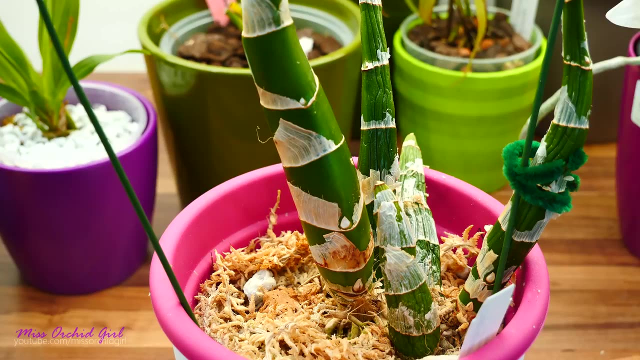 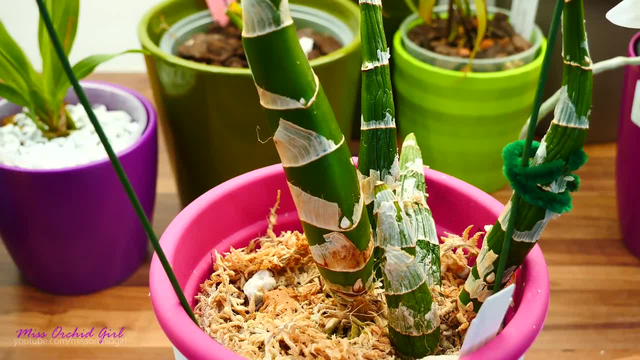 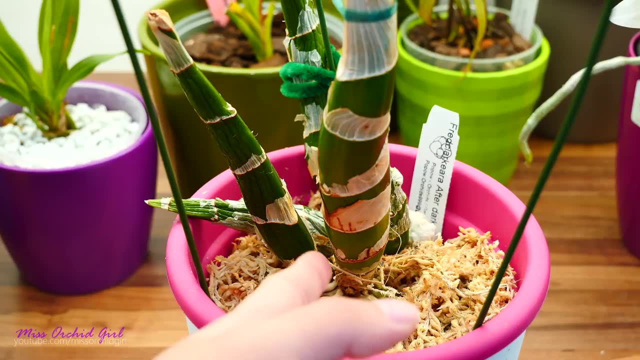 These eyes can also form entire flower spikes, so nut buds. But unlike the phalaenopsis, let's say, we can actually see these eyes And the number of available eyes on the cane can vary depending on the size of the cane And which of these eyes will develop Again. 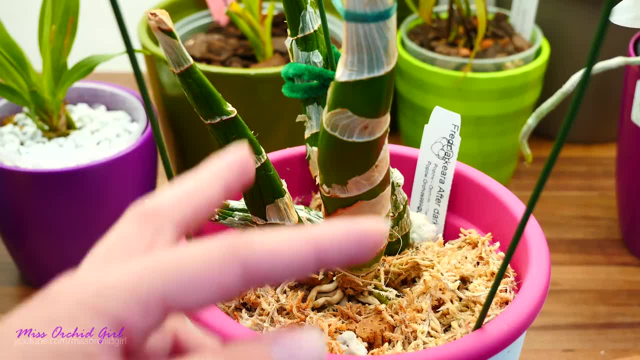 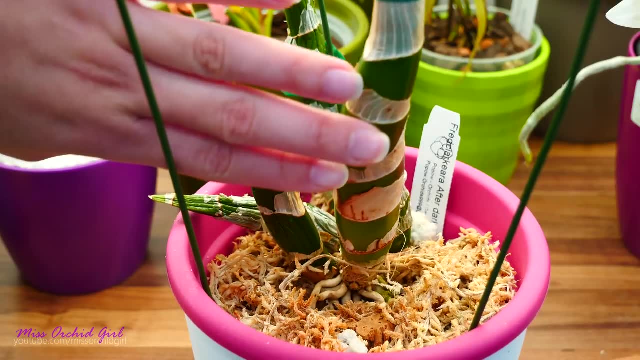 it's kind of up to chance, unless we actively try and propagate it and cut away the pseudobulb, which I don't advise you necessarily to do. but it is actually possible And in my case I think I can see a bottom eye starting to swell up, meaning that this orchid will create. 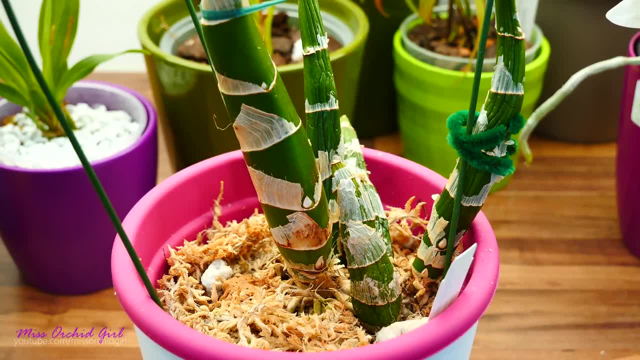 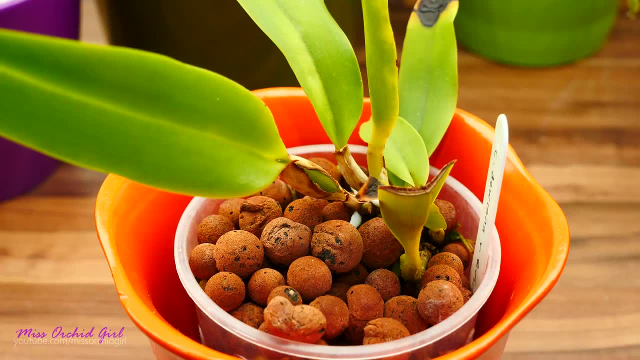 new growth from the base, so these eyes can actually signify something else. depending on the orchid. We can generalize, of course, but there are always exceptions. Typically, cattleya orchids produce new growth from the base. You can see I have a swollen. 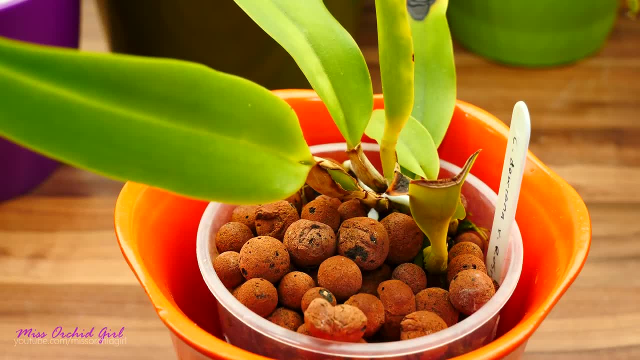 eye here, and they flower on top of each cane. Well, there are exceptions here as well. There are cattleyas which produce flower spikes from the base, And they start out just like a new growth. One of them is the cattleya nobilior, but there 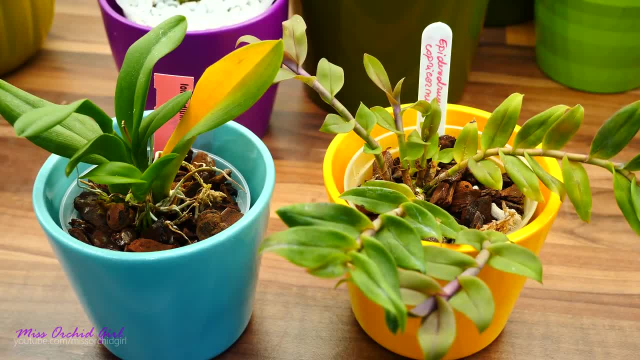 are other cattleyas as well. So bottom line, these eyes you hear people talking about, are nothing more than growth points. They can be called nodes, buds, growth points. All of this is pretty casual talk between orchid growers. As a beginner, all you need to know. 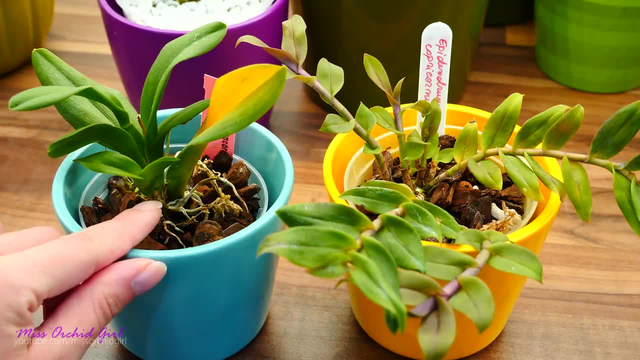